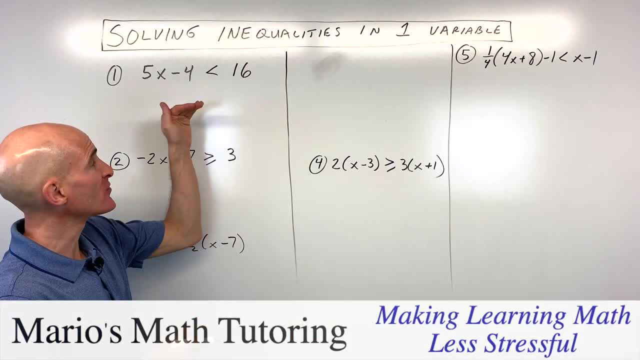 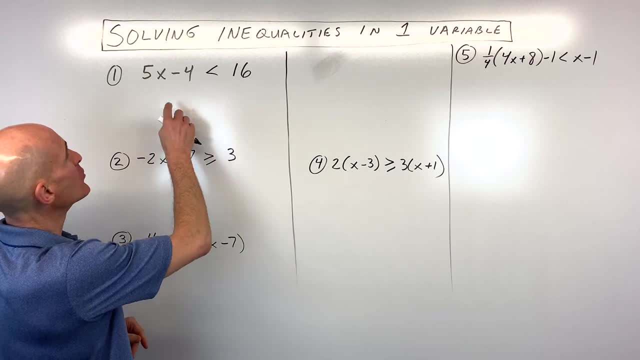 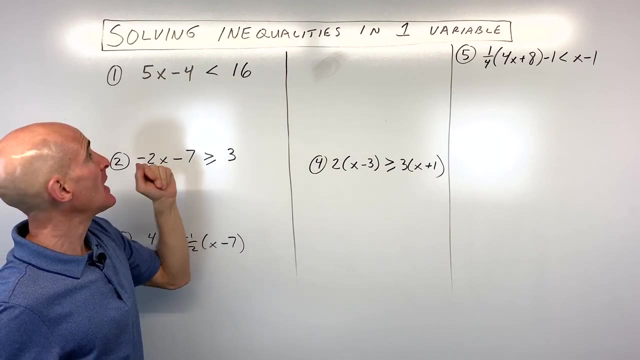 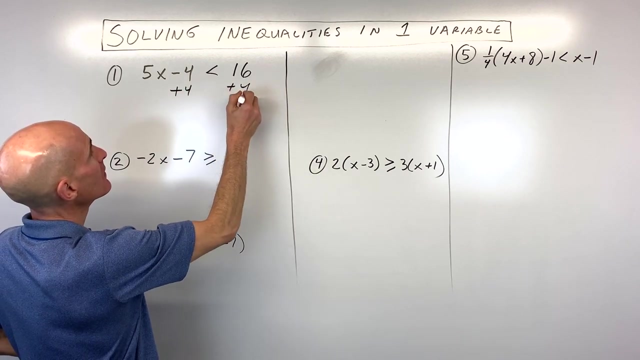 Okay, we're going to go through five inequalities. We're going to start out with some simple ones and get a little bit more challenging as we go through these, See if you can pause the video and do these on your own. The first one: what you want to do when you're solving these inequalities is you want to get the variable by itself on one side of the inequality And ideally you want to get it on the left side. So let's start with this first one. What I'm going to do is I'm going to add four to both sides of the inequality to keep it balanced right. So that's going to give us 20.. And if four negative. 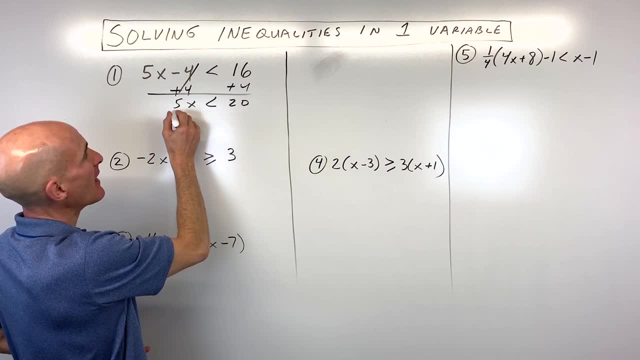 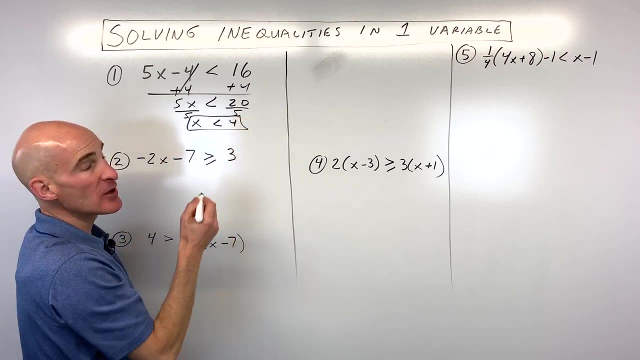 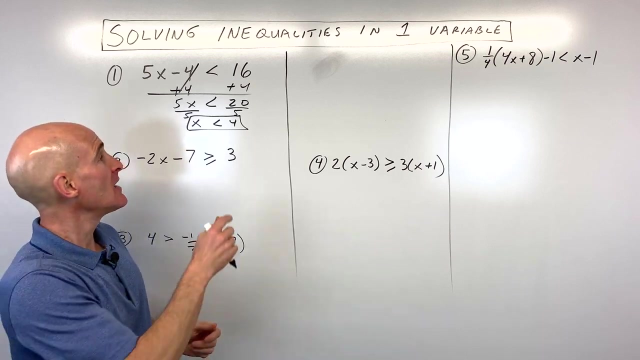 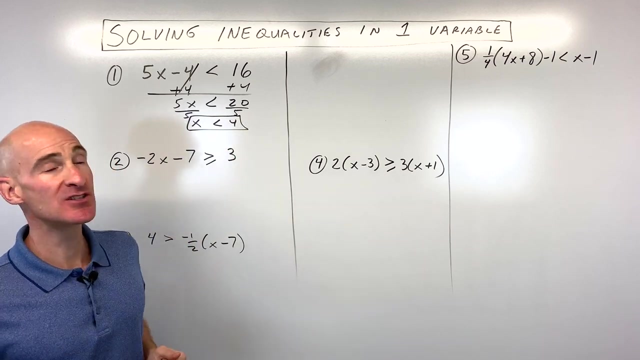 four cancel out. And now what's the opposite of multiplying by five? we want to divide both sides by five And that comes out to x is less than four. Now, one thing you want to be careful of when you're working with inequalities is that if you multiply or divide both sides by a negative number, this inequality sign will change directions- okay, or flip. But in this case we divided by positive five, so it doesn't change direction. Now, when you look at this on the number line, here's four over here. 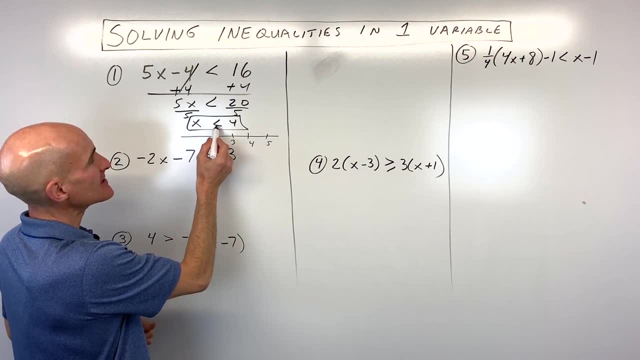 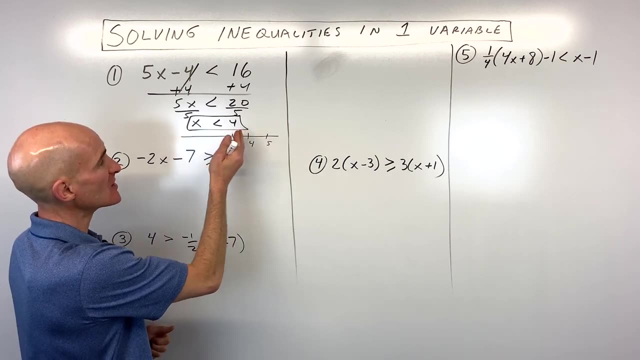 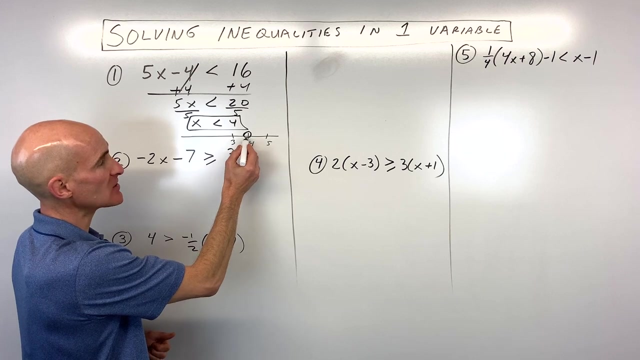 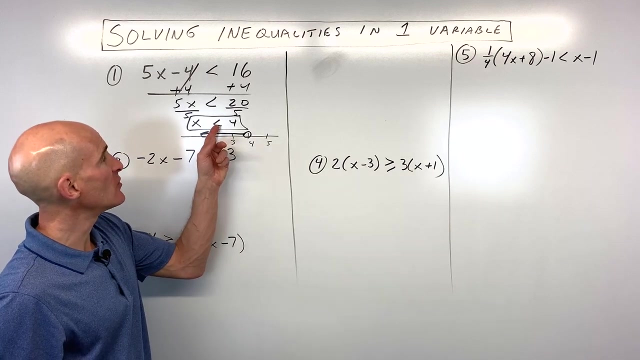 here's five, here's three. see how x is less than four. that means that it can be any value to the left of four on the number line. So as these values get smaller and smaller, so it doesn't equal four, it's just going to be less than four. So we're going to draw this as an open circle. okay, so not including four, and then all the values to the left. One way that students sometimes think about this is that you can think of this when the variables on the left- like this is kind of looks like an arrow. see how it's pointing to the left. So all the values to the left. 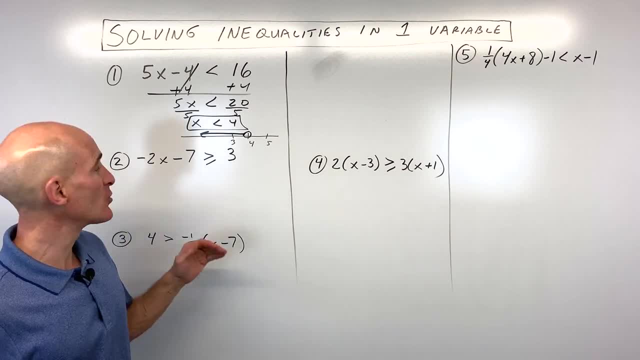 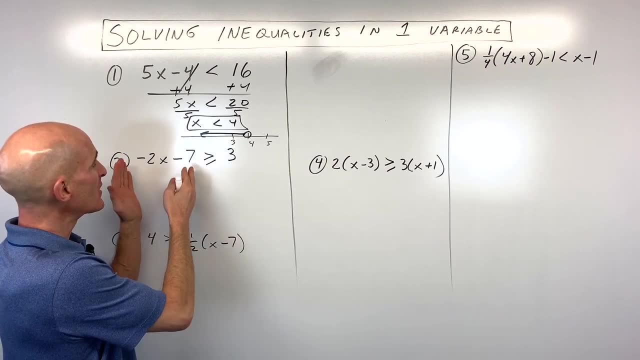 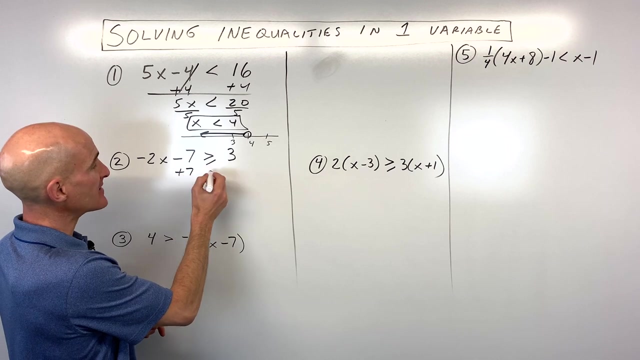 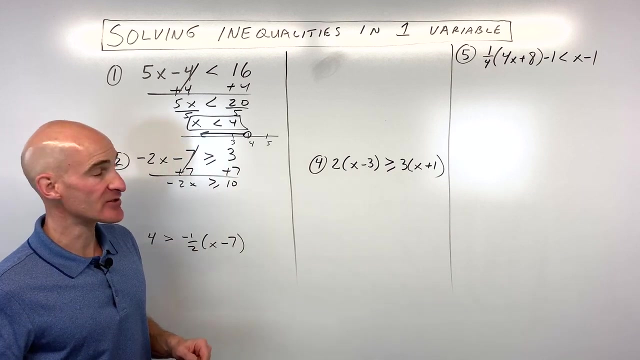 all the values less than four to the left of four. Okay, let's try number two, a little bit more challenging. So this one same idea. we want to get this variable by itself on one side of the inequality, So we can think about working from the outside in towards that variable. So what I'm going to do is I'm going to subtract seven. So I'm gonna do the opposite: I'm going to add seven. Okay, so now we're down to negative two. x is greater than or equal to 10, because the seven and negative seven cancel. The opposite of multiplying by negative two is to divide both sides by negative two. So 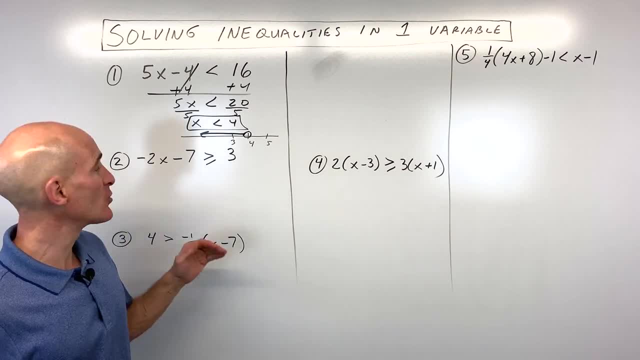 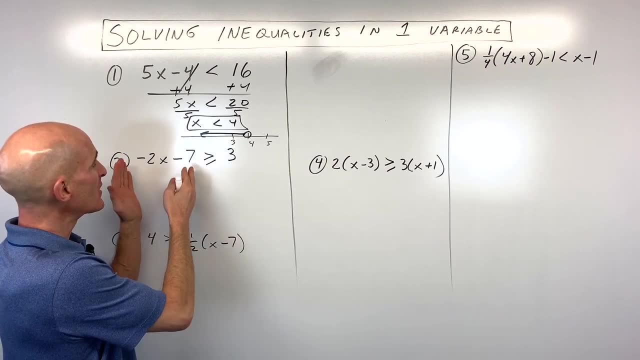 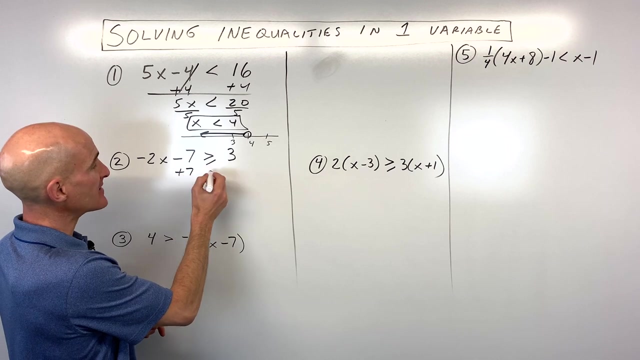 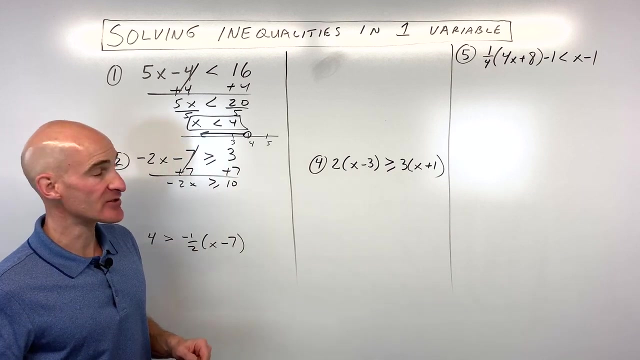 all the values less than four to the left of four. Okay, let's try number two, a little bit more challenging. So this one same idea. we want to get this variable by itself on one side of the inequality, So we can think about working from the outside in towards that variable. So what I'm going to do is I'm going to subtract seven. So I'm gonna do the opposite: I'm going to add seven. Okay, so now we're down to negative two. x is greater than or equal to 10, because the seven and negative seven cancel. The opposite of multiplying by negative two is to divide both sides by negative two. So 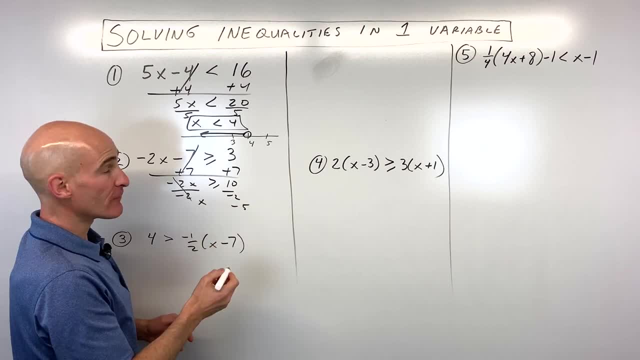 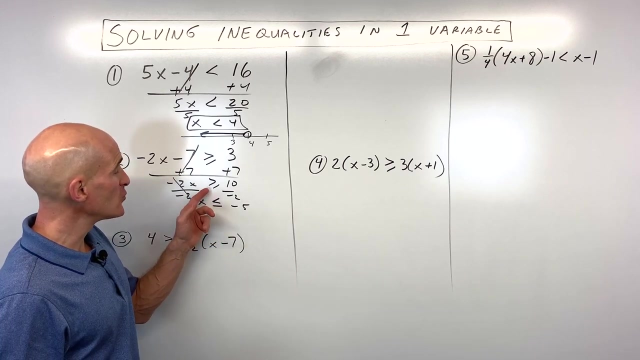 those cancel. And now we're just left with negative five. But look what just happened. I divided both sides by a negative number. this inequality sign is going to change directions, So it's going to be facing the other way. instead of greater than or equal to, it now becomes less than or equal to. one way to remember this to. sometimes students get a bit confused with the greater than and less than. see how this kind of looks like an L tilted, So you can think of like L for less than. And now we're just going to go to the number line. So here's negative five, here this is negative six and this is negative four. 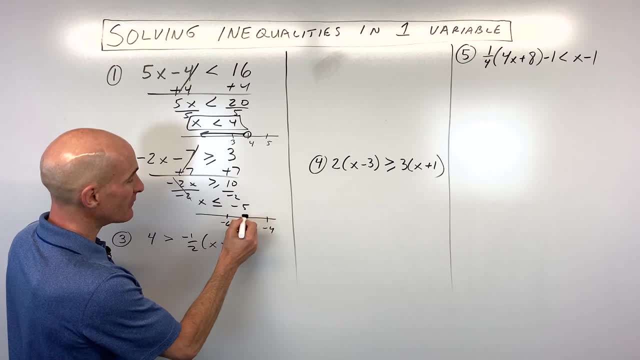 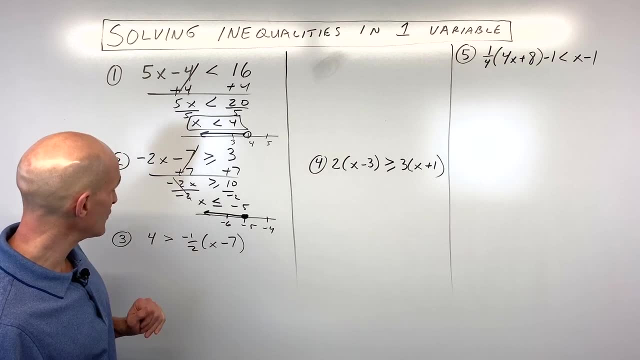 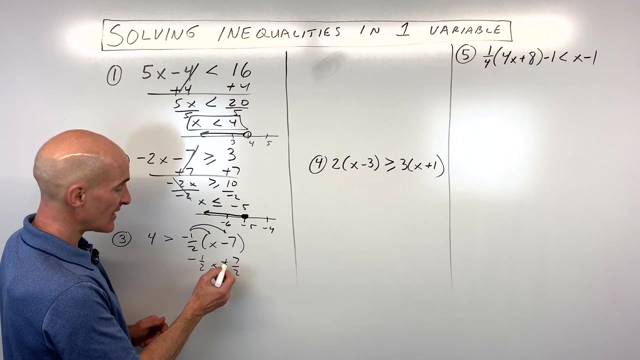 It's less than or equal to. so now, this time it equals negative five. Okay, as well as all the values that are to the left than or less than negative five. Okay, number three: see if we can do this one. This one's a little bit more challenging because we have the variable on the right side. Okay, so let's go see how we're going to approach that one. Let's start by distributing the negative one half, So that's negative one half x plus seven over two, because negative times a negative is a positive, And we've got four on the left here still. Now, what I'm going to do here, because I have 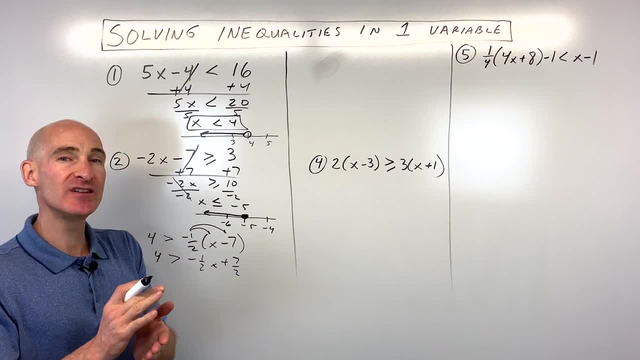 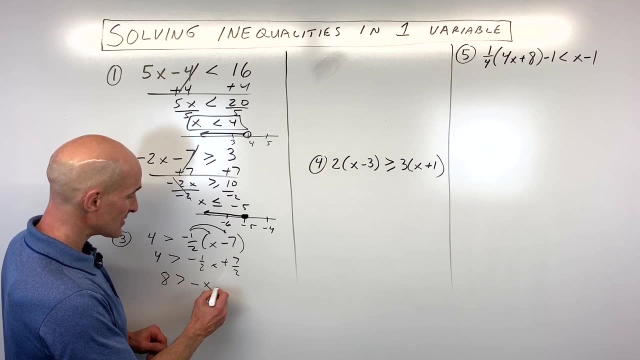 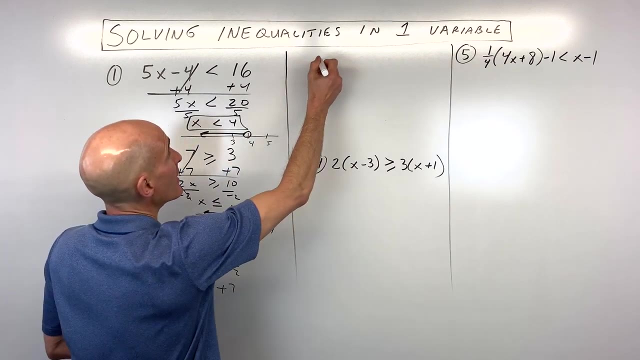 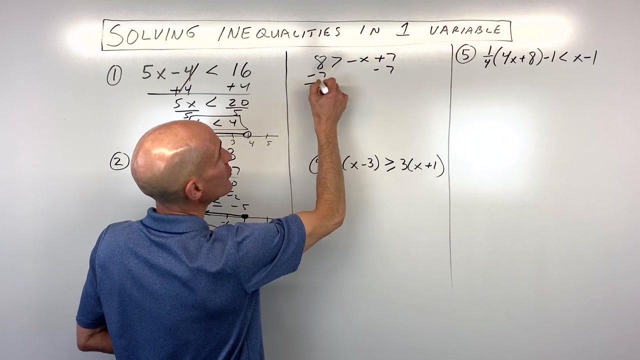 these fractions is I'm going to multiply everything by two to clear the denominators, to get rid of those fractions. So if I multiply everything by two, that gives us eight is greater than negative one, x plus seven. And then let's continue this on over up here. I'm going to rewrite it So we have eight is greater than negative x plus seven. And then instead of adding seven, I'm gonna do the opposite. I'm going to subtract seven from both sides, So that's one is greater than negative x. I'm going to get the x by itself. 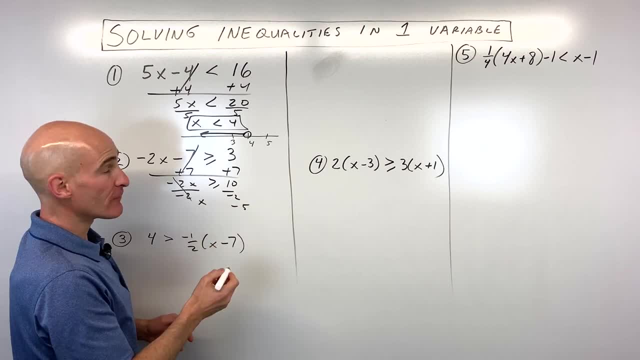 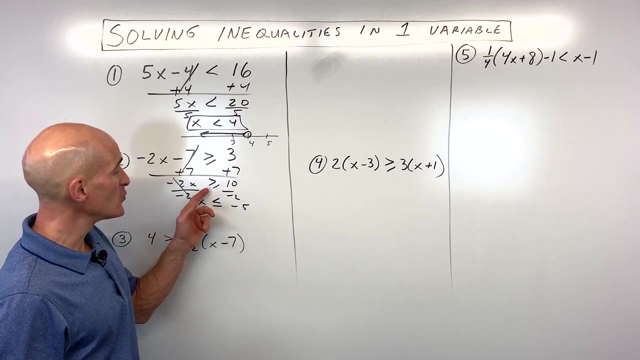 those cancel. And now we're just left with negative five. But look what just happened. I divided both sides by a negative number. this inequality sign is going to change directions, So it's going to be facing the other way. instead of greater than or equal to, it now becomes less than or equal to. one way to remember this to sometimes students get a bit confused with the greater than and less than. See how this kind of looks like an L tilted, So you can think of like L for less than. And now we're just going to go to the number line. So here's negative five, here This is negative six And this is negative four. And 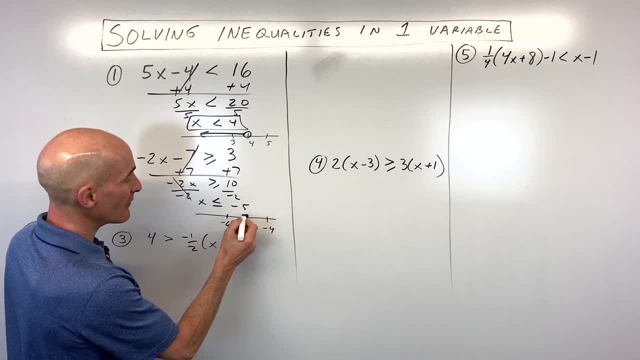 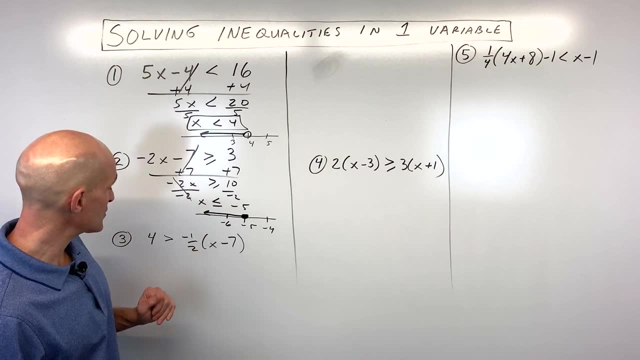 it's less than or equal to. so now, this time it equals negative five, okay, as well as all the values that are to the left, then. or less than negative five- Okay, number three: see if we can do this one. This one's a little bit more challenging. 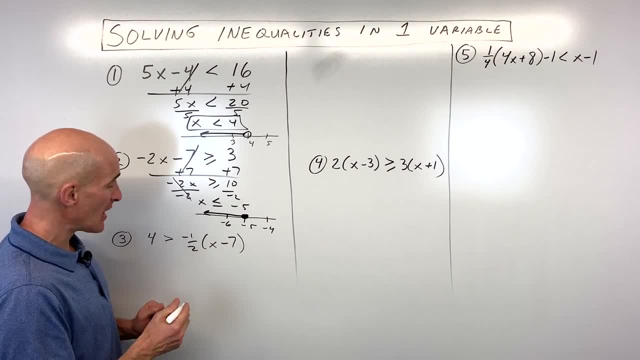 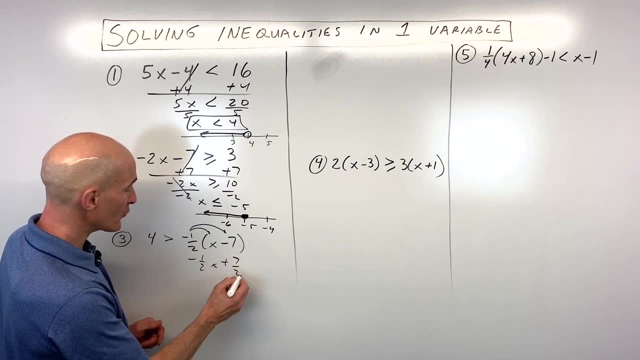 because we have the variable on the right side. okay, so let's go see how we're gonna approach that one. Let's start by distributing the negative 1 1⁄2, so that's negative 1 1⁄2x plus seven over two. 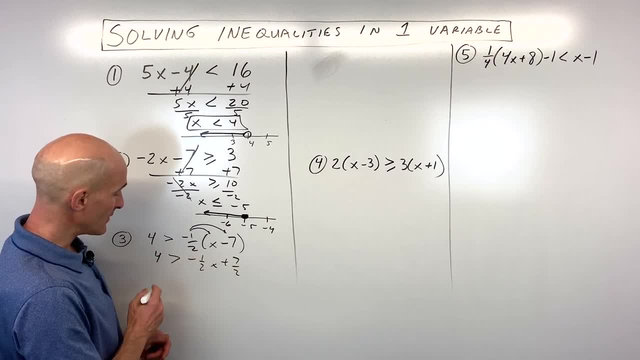 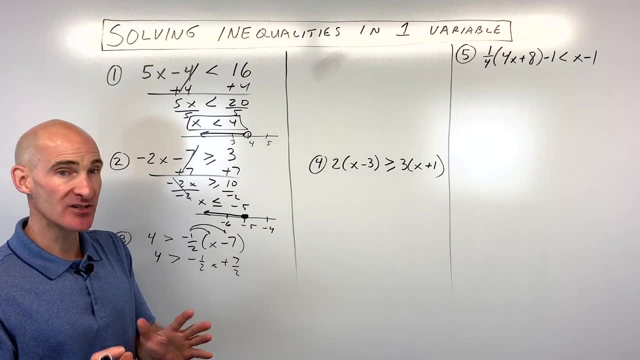 because negative times, a negative is a positive and we've got four on the left here still. Now what I'm gonna do here, because I have these fractions, is I'm gonna multiply everything by two to clear the denominators, to get rid of those fractions. 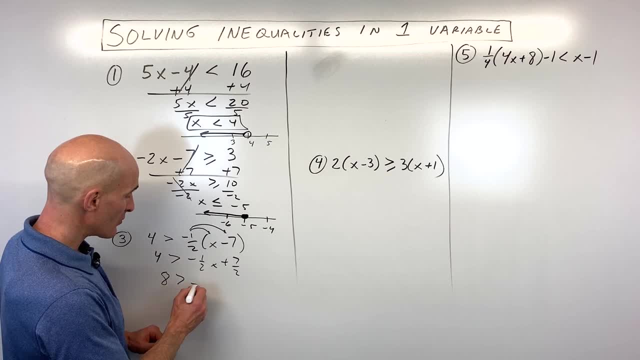 so if I multiply everything by two, that gives us eight is greater than negative 1x plus seven. and then let's continue this on over up here. I'm going to rewrite it. so we have: eight is greater than negative x plus seven. 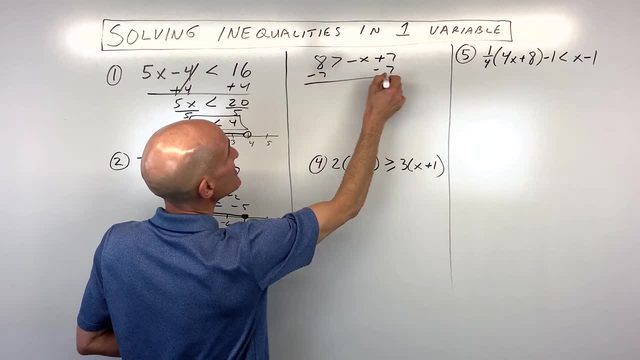 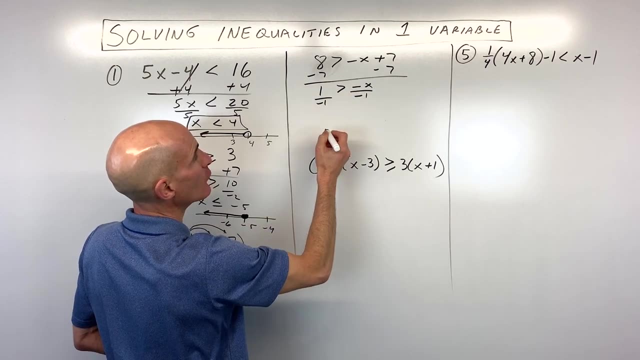 and then, instead of adding seven, I'm gonna do the opposite. I'm gonna subtract seven from both sides, so that's one is greater than negative x. I'm gonna get the x by itself by dividing both sides by negative one, so now we have x and negative one. 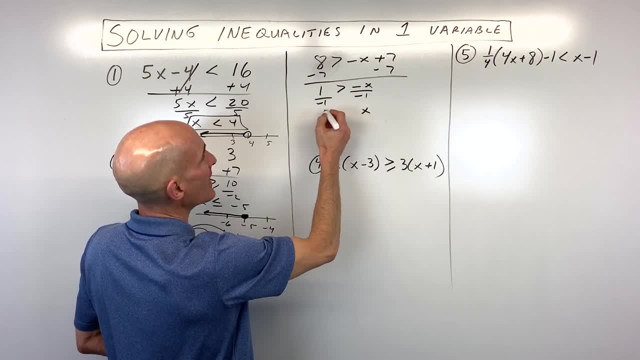 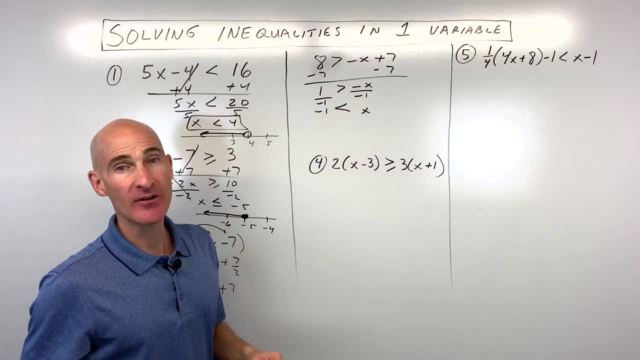 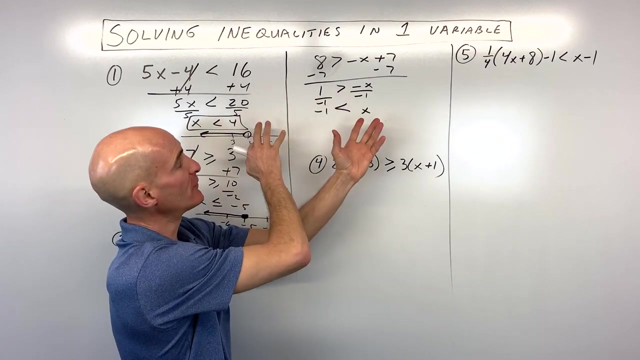 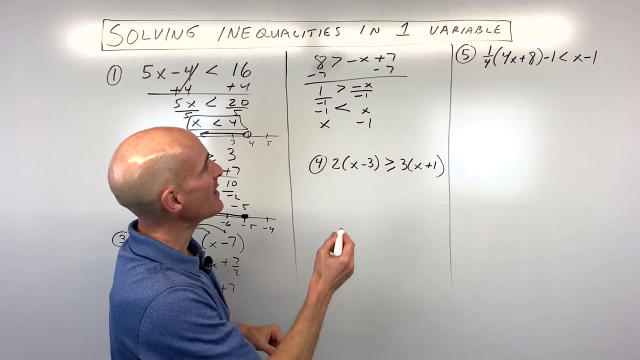 by dividing both sides by negative one. So now we have x and negative one, But look what just happened. I multiplied, or divided both sides by a negative number. this inequality changes direction right, But we also have the variable on the right. we want to really get the variable on the left. So what I'm going to do is I'm going to pick up this whole inequality, I'm going to flip it over, And so this is going to be x negative one. see how this is opening towards the x. okay, like that, it's still going to be opening towards the x. Okay, so I just took the whole thing, I flipped it over. 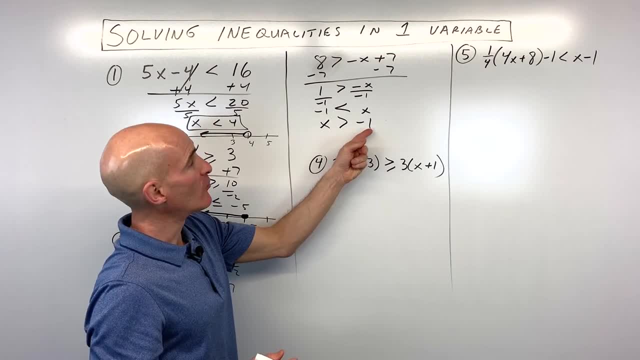 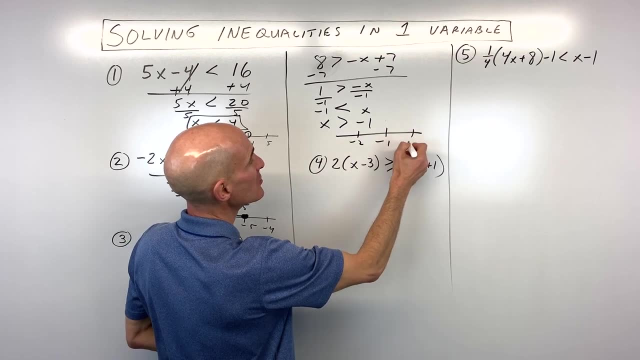 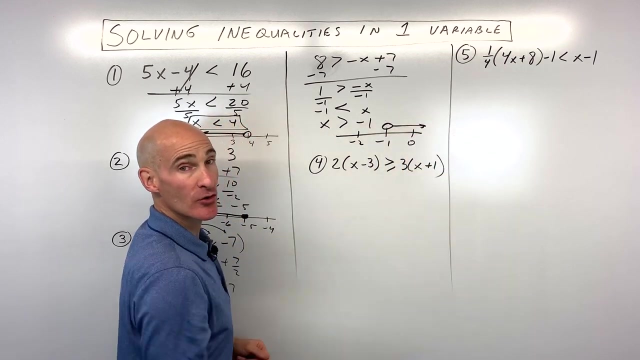 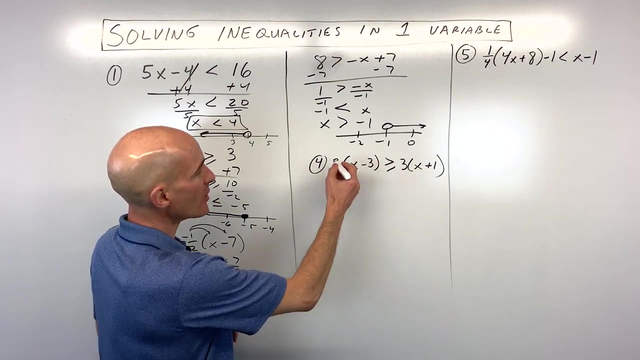 x is greater than negative one. Or if you read this from right to left, this is like negative one is less than x. Now we can go ahead and graph it. So here's negative one, here's negative two, here's zero. we want all the values that are greater than, but not including negative one. So greater than, we're going to the right. so all the values that are greater. Okay, number four, a little bit more challenging this one. we've got variables on both sides of the inequality. I'd start by distributing the two, So that gives us two x minus six. distribute the. 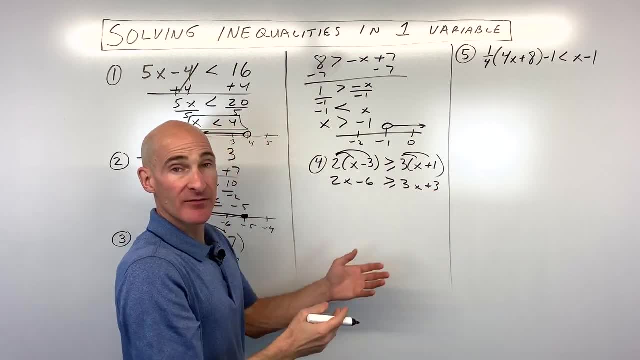 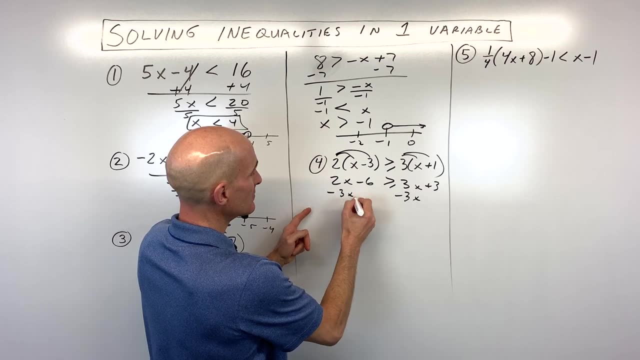 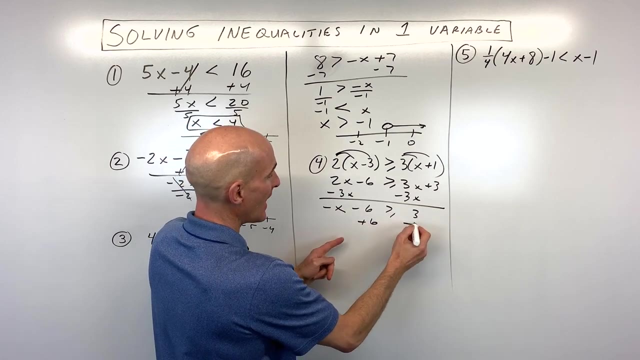 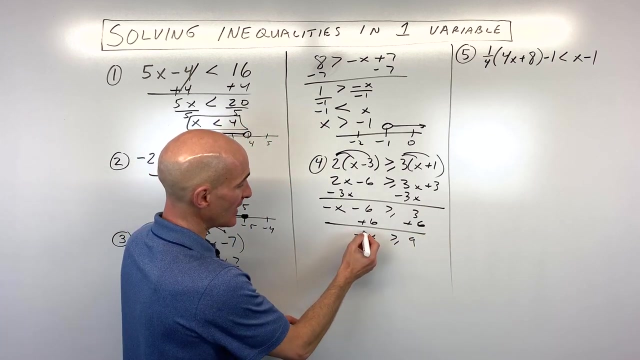 three, that's three x plus three. And now we want to get the variables on one side, numbers on the other, just like solving an equation. So what I'm going to do here is I'm going to subtract three x from both sides, So that gives us negative one x. And then, instead of subtracting six, I'm going to add six to both sides, So that comes out to nine. But we have a negative x which is like a negative one x. we're going to divide both sides by negative one. And remember when you multiply or 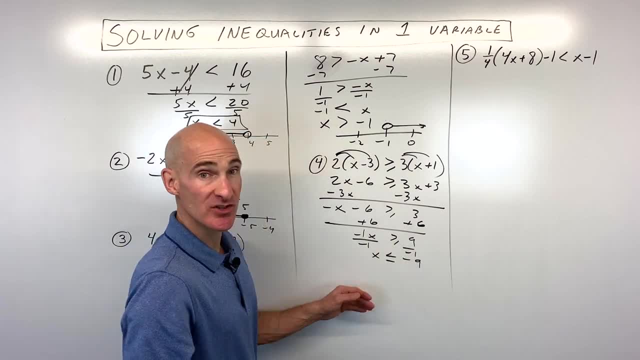 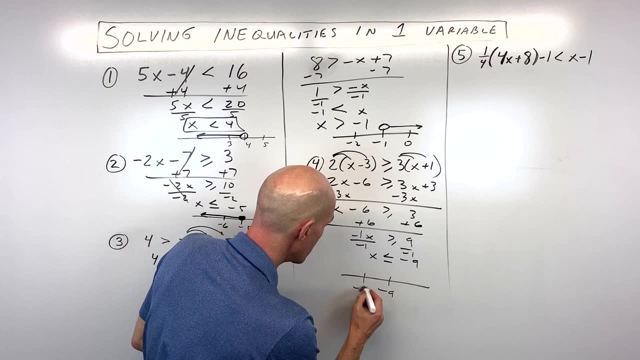 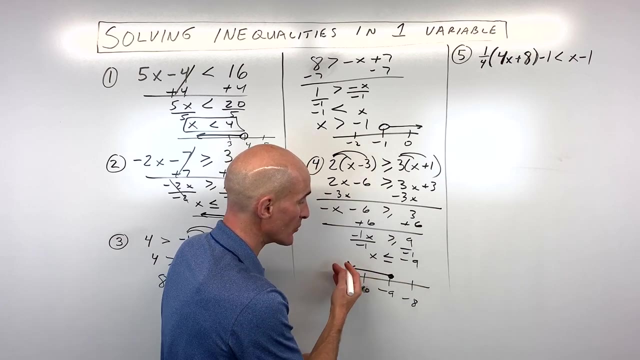 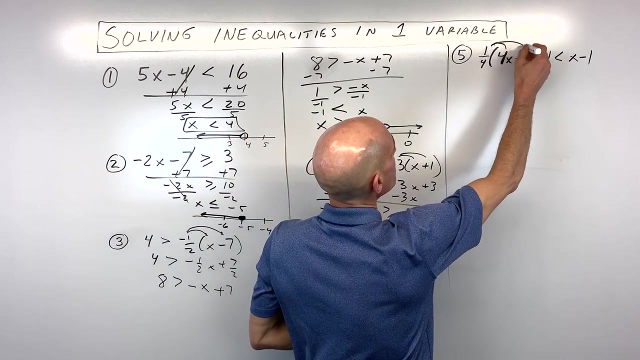 divide, you're going to get a negative one, x. So we're going to divide both sides by negative one. And remember when you multiply or divide by a negative number, that inequality sign changes directions. So we have x is less than or equal to negative nine, and we have negative nine, negative 10 over here and negative eight over here. and x is less than or equal to, so it includes negative nine as well as all the values less than or to the left of negative nine. Okay, number five. last problem: see if we can do this one Here, we're going to distribute the one. fourth, And one thing when you're working with fractions it makes it a little bit easier is to put the whole numbers over one, because 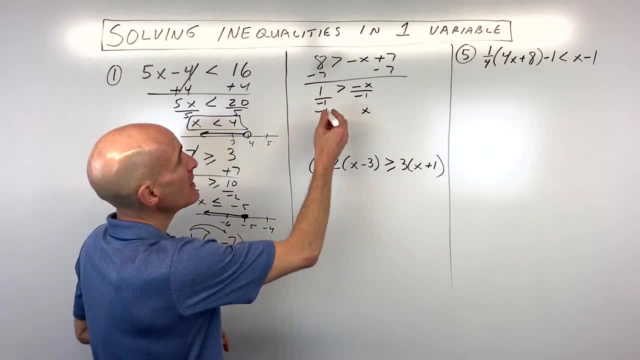 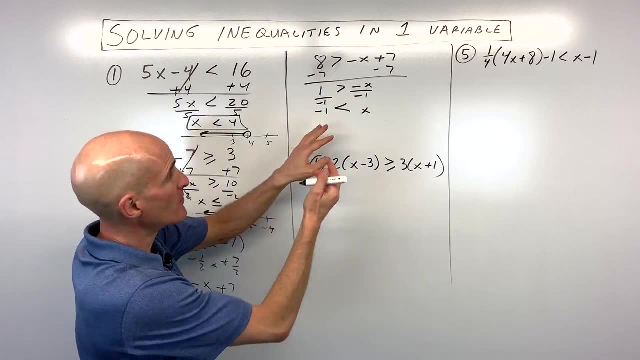 but look what just happened. I multiplied, or divided both sides by a negative number. This inequality changes direction right, but we also have the variable on the right. We wanna really get the variable on the left. so what I'm gonna do is I'm gonna pick up. 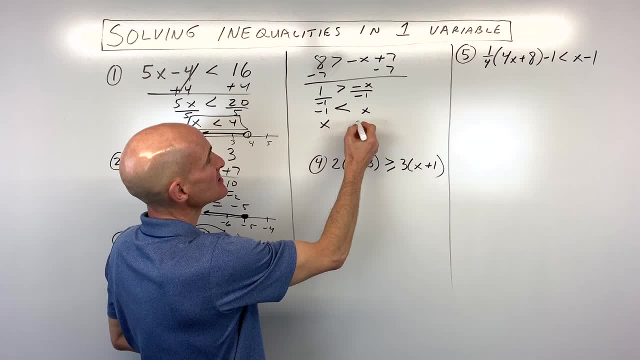 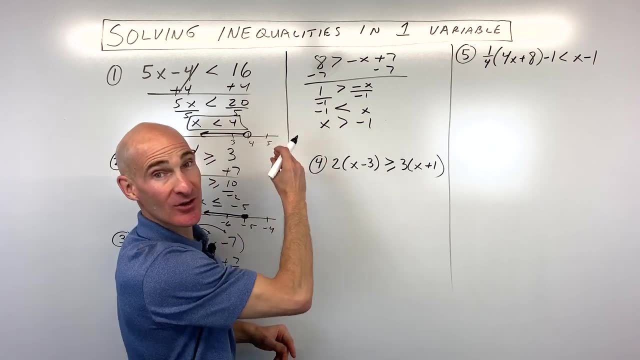 this whole inequality, I'm gonna flip it over and so this is gonna be x negative. one See how this is opening towards the x. okay, like that It's still gonna be opening towards the x. okay, so I just took the whole thing. 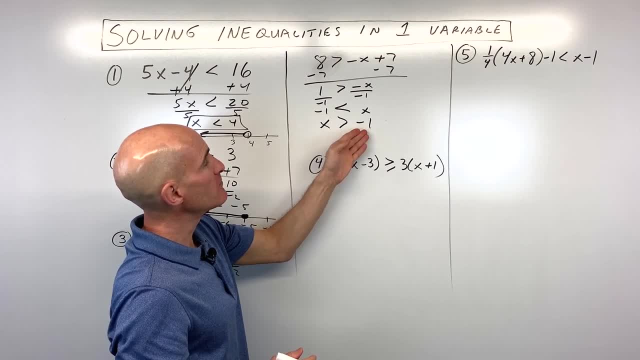 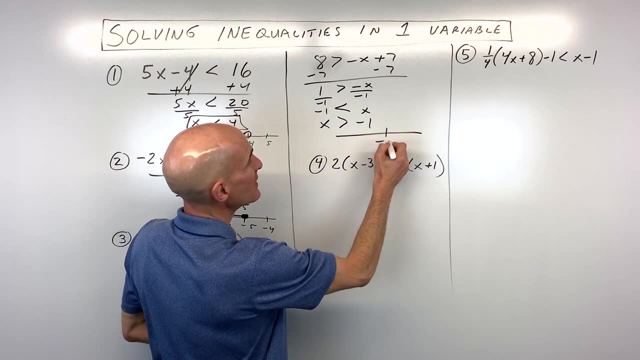 I flipped it over: X is greater than negative one. or if you read this from right to left, this is like negative one is less than x. Now we can go ahead and graph it. so here's negative one, Here's negative two. 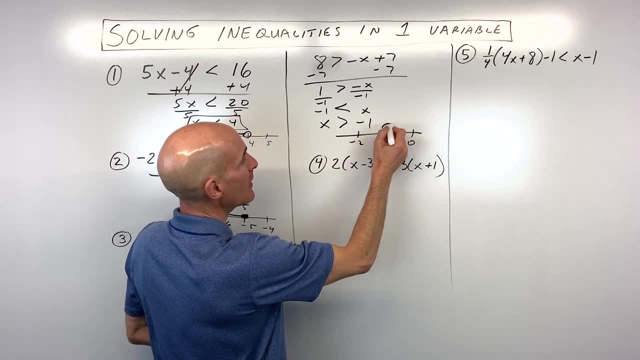 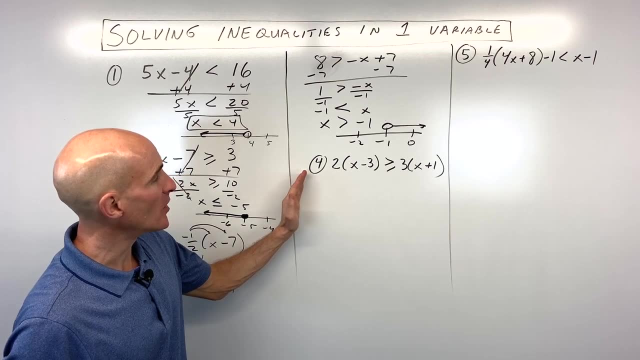 Here's zero. We want all the values that are greater than, but not including negative one. so greater than, we're going to the right. so all the values that are greater. Okay, number four, a little bit more challenging, this one. 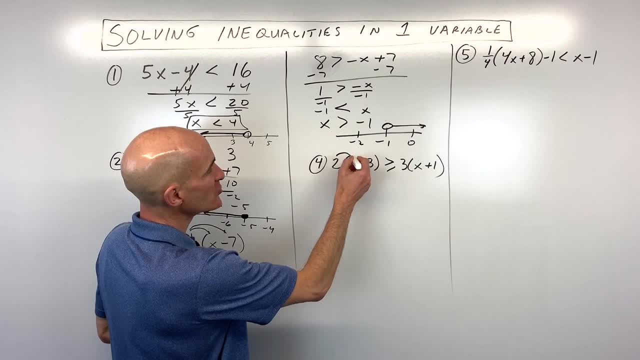 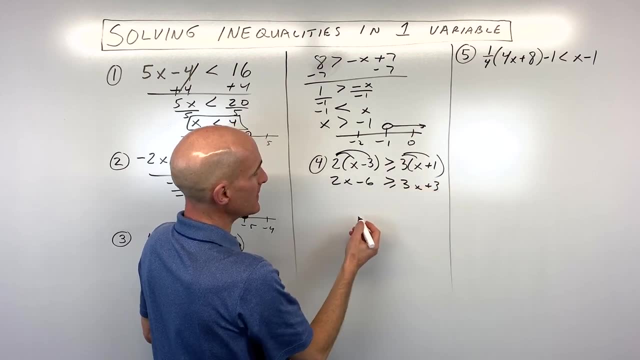 We've got variables on both sides of the inequality. I'd start by distributing the two, so that gives us two x minus six. Distribute the three, That's three x plus three. and now we want to get the variables on one side. 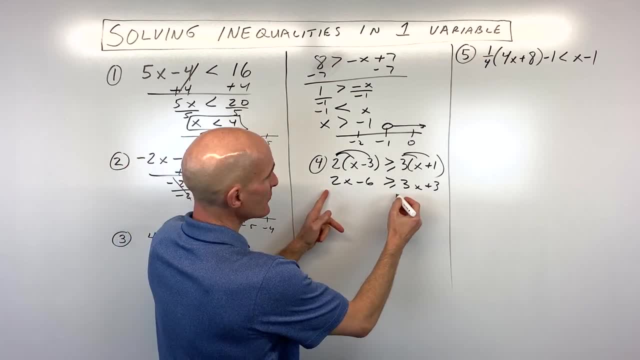 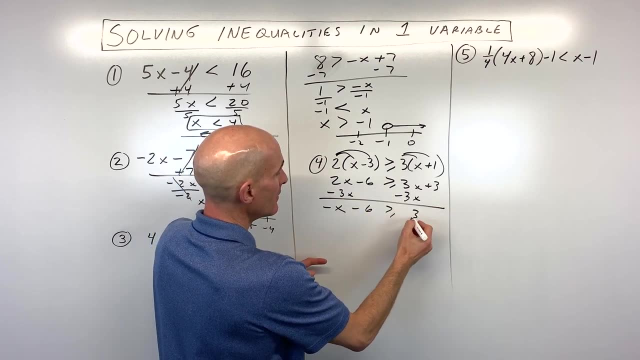 and numbers on the other, just like solving an equation. so what I'm gonna do here is I'm going to subtract three x from both sides, so that gives us negative one x, and then, instead of subtracting six, I'm going to add six to both sides. 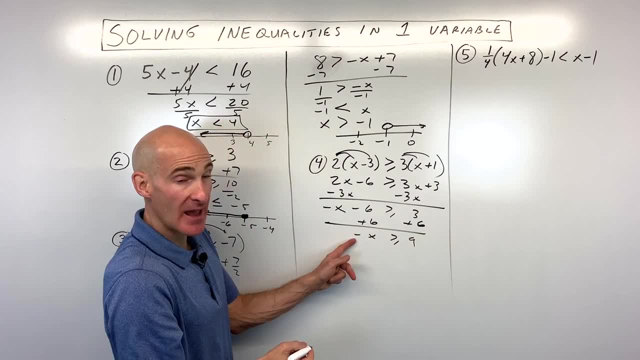 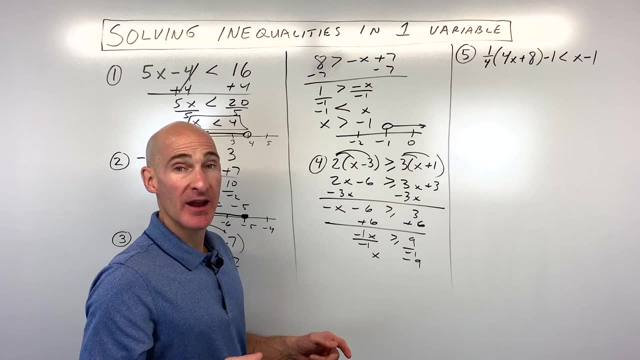 so that comes out to nine. but we have a negative x, which is like a negative one x. so we're gonna divide both sides by negative one and remember, if we multiply or divide by a negative number, that inequality sign changes directions. 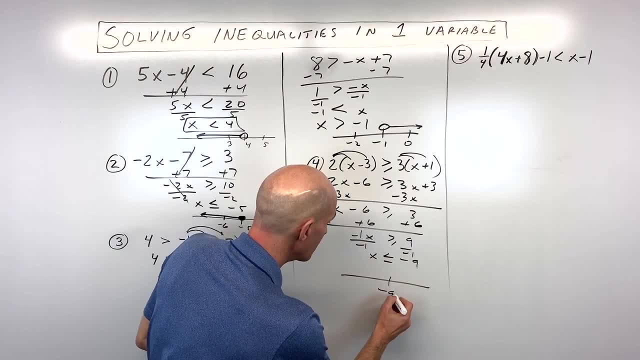 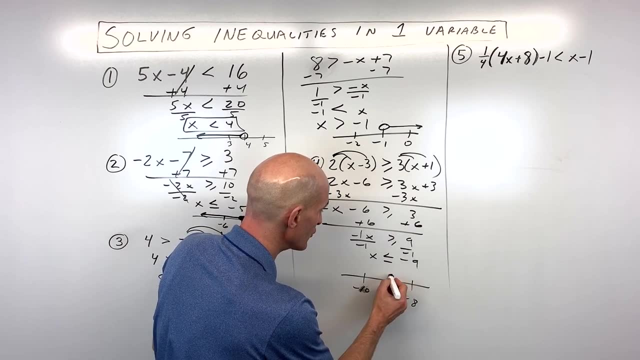 so we have x is less than or equal to negative nine, and we have negative nine, negative 10 over here and negative eight over here, and x is less than or equal to, so it includes negative nine as well as all the values less than. 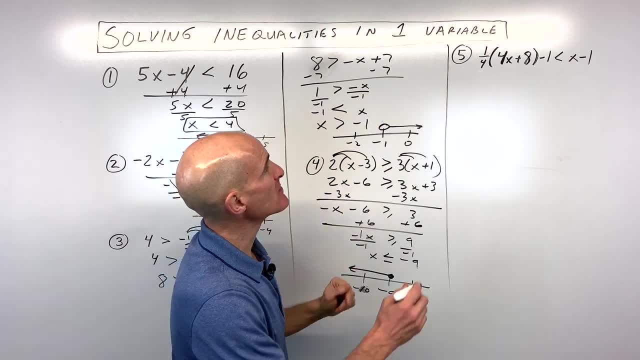 or to the left of negative nine. Okay, number five. last problem, See if we can do this one Here. we're gonna distribute the 1, 4th. and one thing: when you're working with fractions, that makes it a little bit easier. 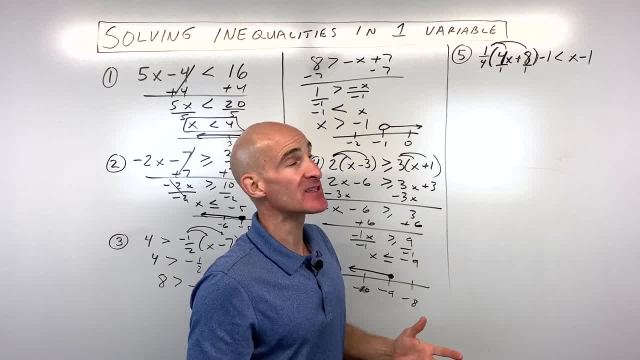 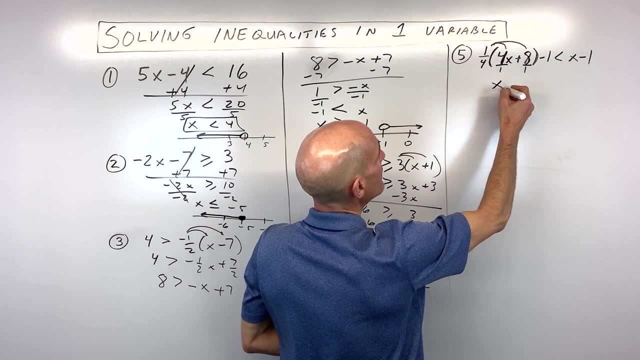 is to put the whole numbers into one, because anything divided by one is itself. and what you can do is you can multiply the numerators together, the denominators together, so that gives us four over four, which is one. and then here we have one times eight is eight. 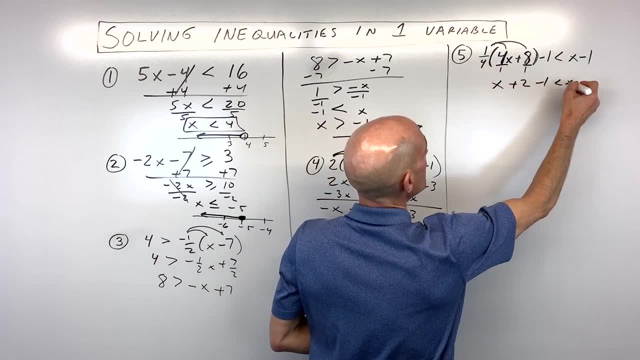 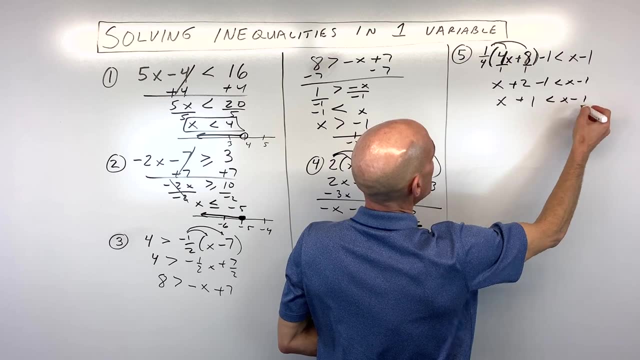 four times one is four, eight divided by four is two, and that's an easier way to work with fractions and whole numbers. and then now let's just combine like terms: Two minus one is one, and let's subtract x from both sides. 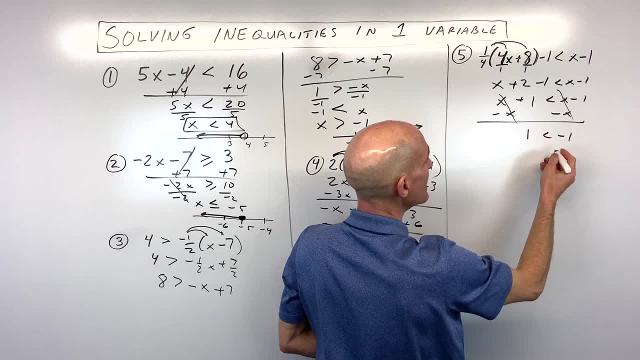 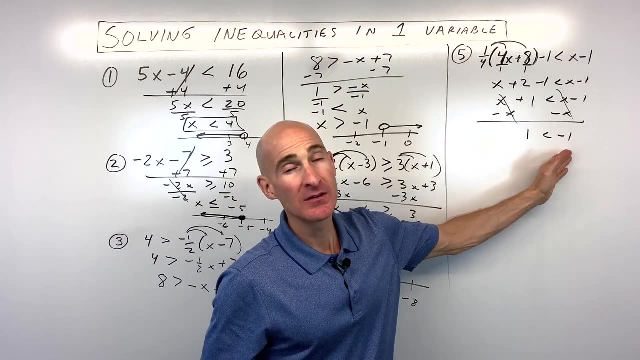 of the inequality. so those cancel and we get: one is less than negative one. Now what happened to our variable? It just rolled on on both sides right And look what we're left with. Is one less than negative one? No, so that means that there's no solution to this problem. 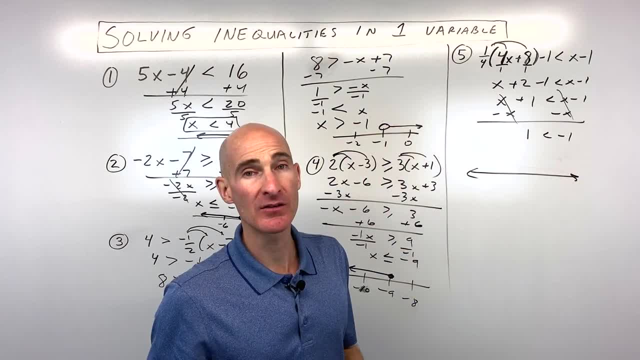 and if you were graphing this on the number line, you would just leave that number line blank, because there's nothing that makes this true. Now, if it was the other way, where one was greater than negative one, that's always true. 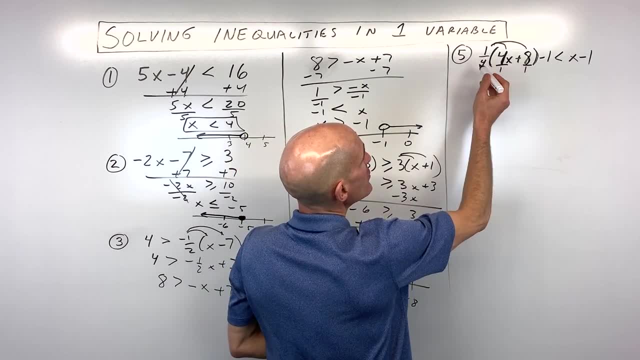 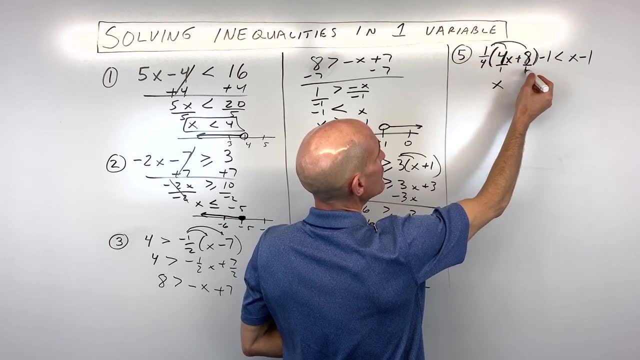 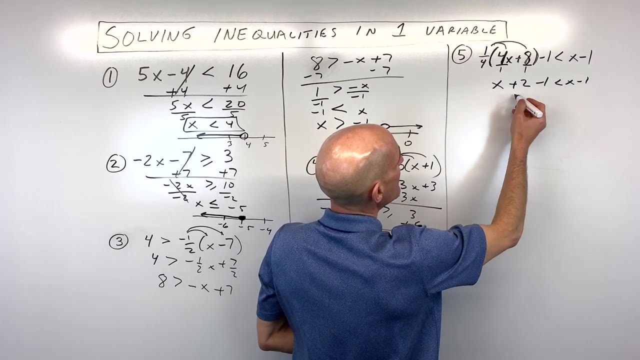 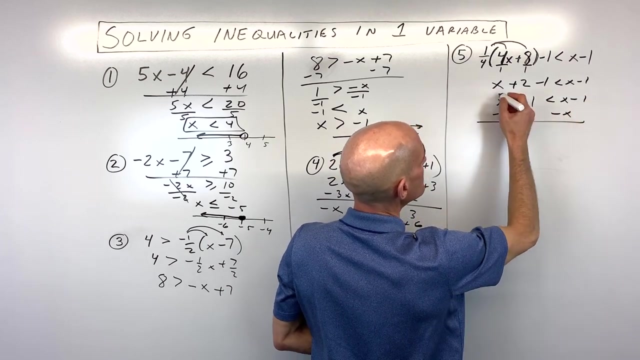 anything divided by one is itself, And what you can do is you can multiply the numerators together, the denominators together, So that gives us four over four, which is one. And then here we have: one times eight is eight. four times one is four. eight divided by four is two, And that's an easier way to work with fractions and whole numbers. And then now let's just combine like terms: two minus one is one And let's subtract x from both sides of the inequality, So those cancel and we get one is less than negative one. Now what happened to our variable? it canceled out on both. 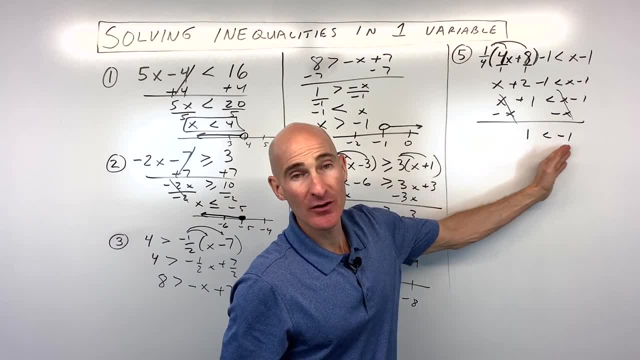 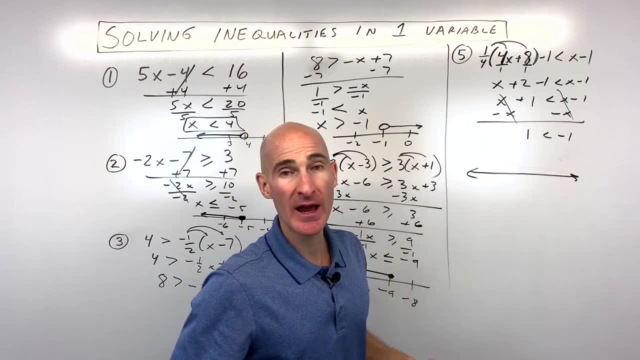 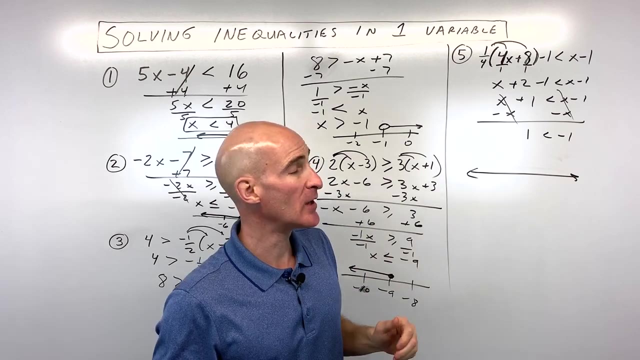 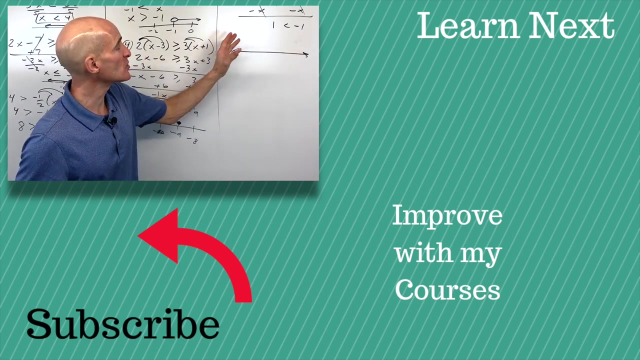 sides right And look what we're left with. is one less than negative one? No, So that means that there's no solution to this problem. And if you were graphing this on the number line, you would just leave that number line blank. okay, because there's nothing that makes this true. Now, if it was the other way, where one was greater than negative one, that's always true And it would be all real numbers And you could then shade or graph. you know the entire number line because it's infinitely many solutions. So these are special cases when the variable cancels out. If you want to see more pre algebra topics, 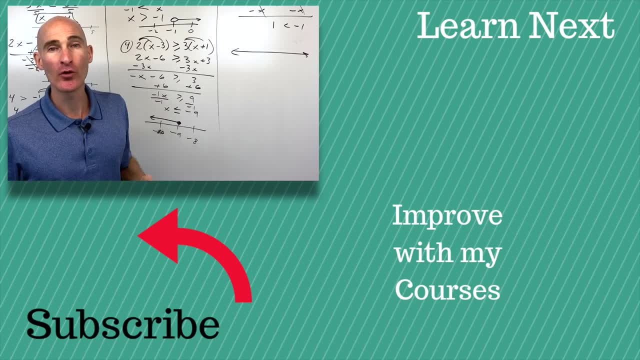 check out my giant pre algebra review where I go through inequalities as well as a lot of other pre algebra concepts in that video right there. I'll see you over in that video. 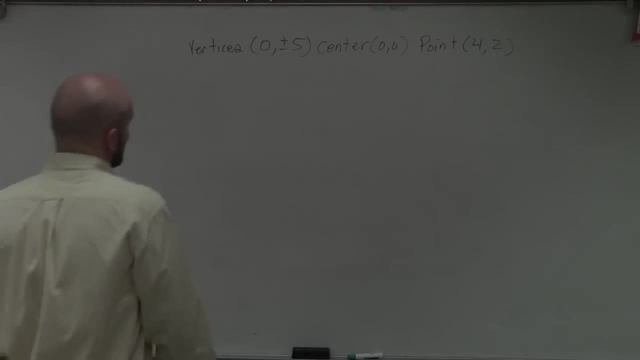 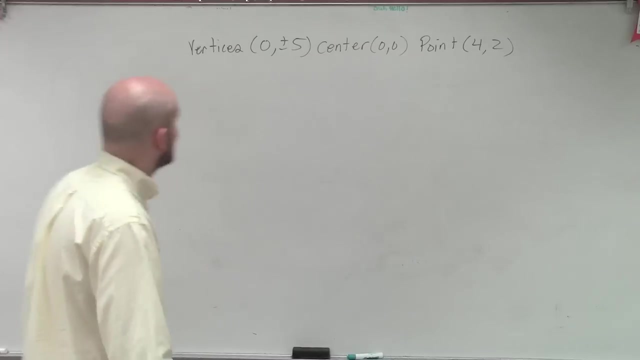 For this problem. what they want us to do is find the right or write the standard form of the equation. So when looking at this, first of all we need to determine if it's going to be horizontal or vertical. So, again, what I like to do is just kind of plot the 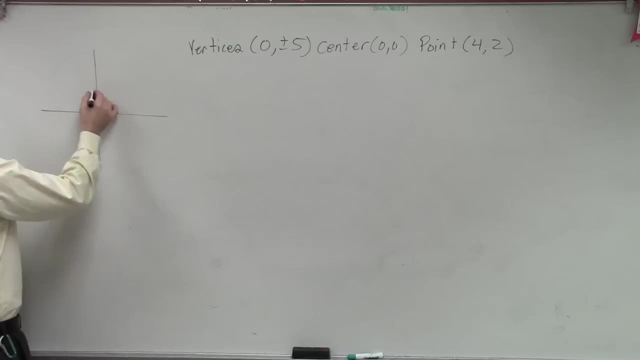 points. My vertices are at zero plus five and zero negative five. So, ladies and gentlemen, am I going to have a vertical or a horizontal Vertical Vertical right? So, therefore, I know now exactly the formula that I'm going to have to use, which is going to be x minus.